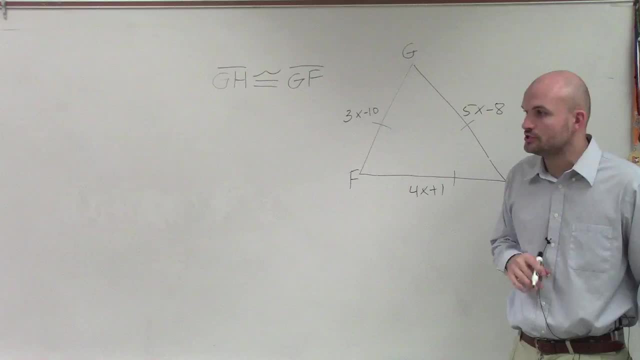 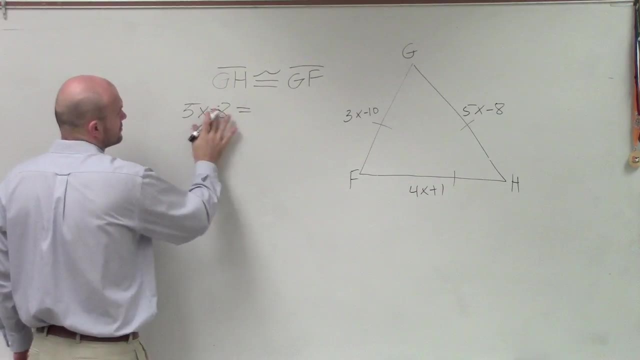 So you have to be able to label them with the two points. So gh is congruent to gf. That means that gh, which is 5x minus 8, is equal in measure, is equal to measure in gf, which is 3x minus 10.. 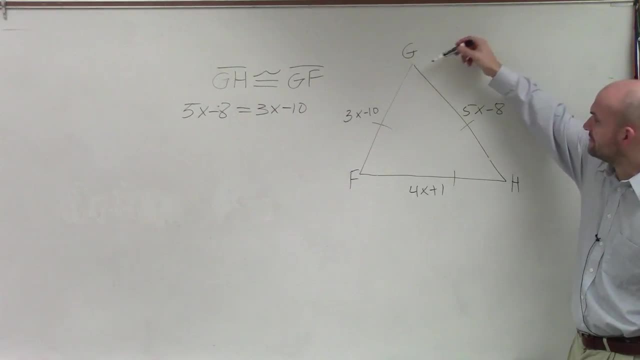 3x minus 8, 5x minus 8 is the measure of gh. I'm sorry. 5x, 5x, 5x, 5x, 5x You're, And the problem is plus 10?. 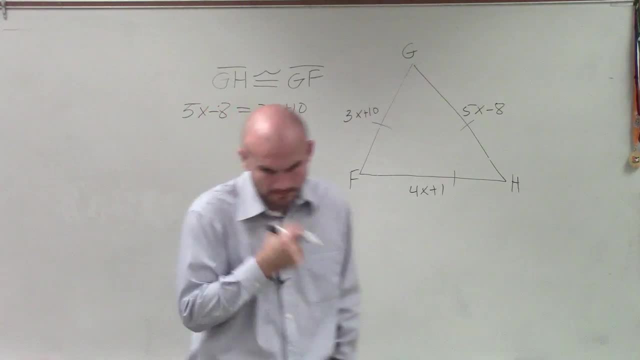 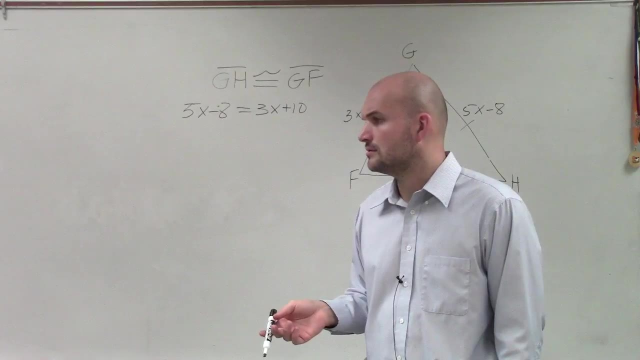 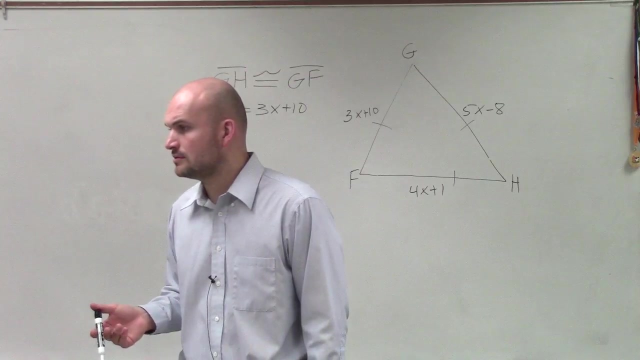 OK, Aidan, you need to be writing this time, Shane. Oh, Keith, do you have a sheet of paper that Shane might be on the phone? No, I don't need a piece of paper, I need a gun. You do need a piece of paper. 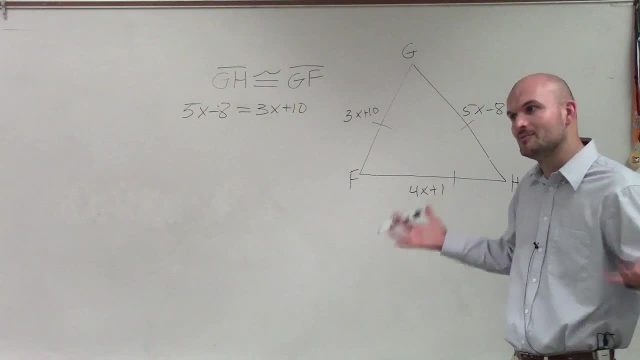 There you go, See, See how helpful people are. You guys are like a community. There you go, All right, so now we've got to solve for x. Now, when we're solving for x, ladies and gentlemen, we have an x on both sides. 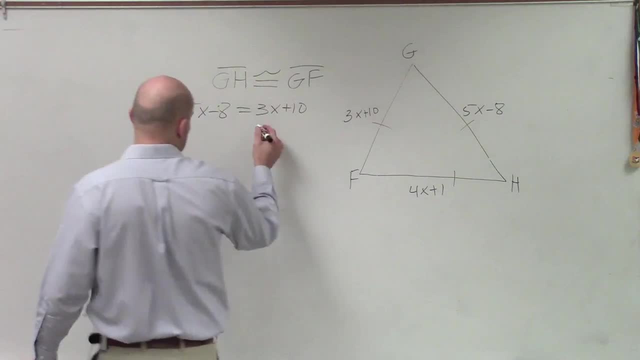 We need to get the variables to the same side. So what I'm going to do is I'm going to subtract a 3x on both sides. What that allows me to do is that adds up to 0x, which is just 0.. 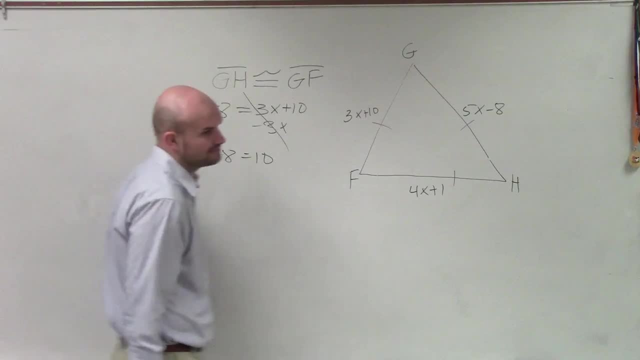 So I'm left with 2x minus 8 equals 10.. Now what I can do is apply my inverse operations to solve for x. So now I'm going to isolate my variable. So to do that, I undo what's happening to the variable. 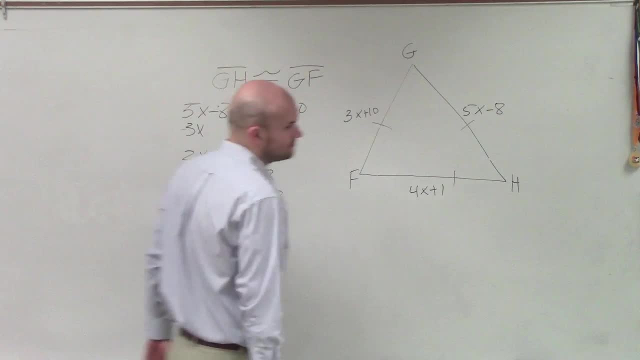 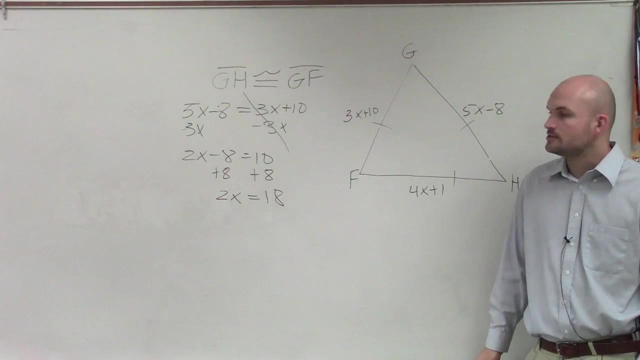 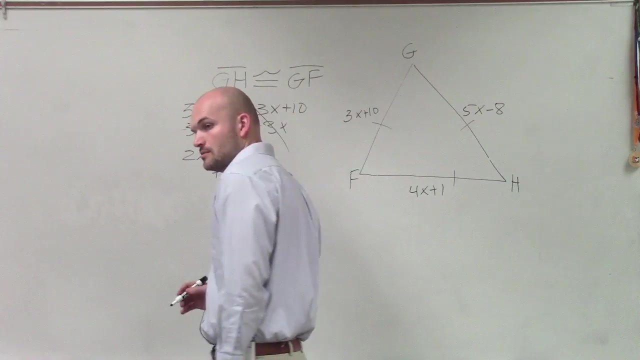 So I add an 8 onto both sides. I have a 3x. Okay, Yeah To x equals 8.. And now what I'll do is I'll divide by dose: x equals 9.. So x equals 9.. 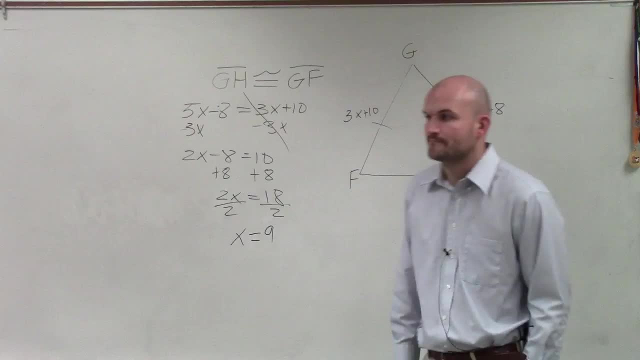 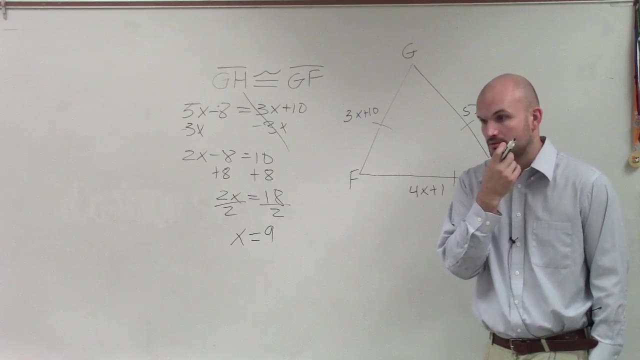 So x equals 9.. Keith, you can go and sit back there if that's helpful for you. I think it really might be. So that's it now, but that's not the question. The question didn't say just find the value of x. 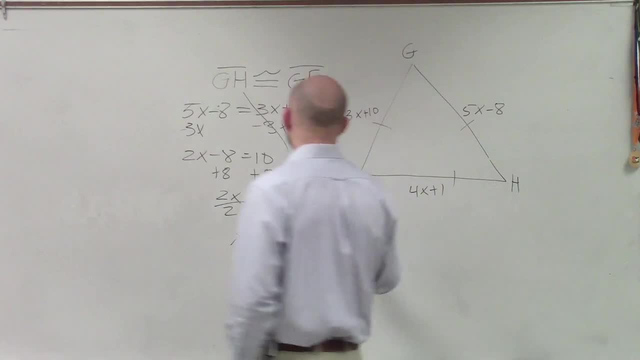 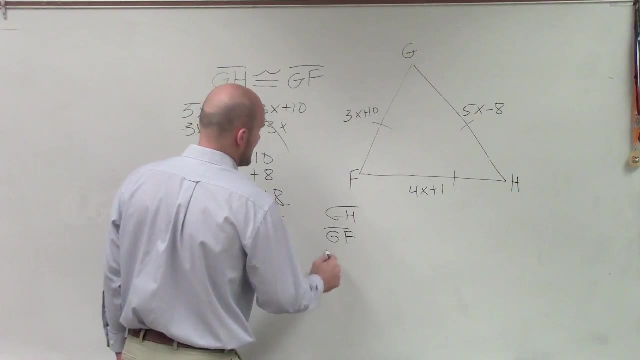 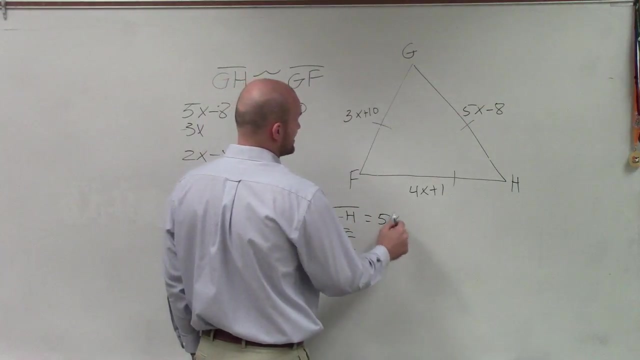 It said, find the value of x and then find the length of each of these sides. So, therefore, we still need to be able to figure out what is gh, what is gf and what is fh. So we know gh is in the formula of 5x minus 8.. 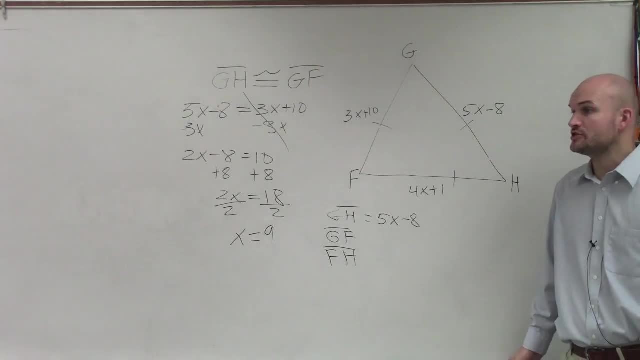 It's gh, It's okay. Shane can move too if he has a problem with it. Yeah, he might. He might have to, It's okay. It's okay, We understand. I know, I know some people have a hard time. 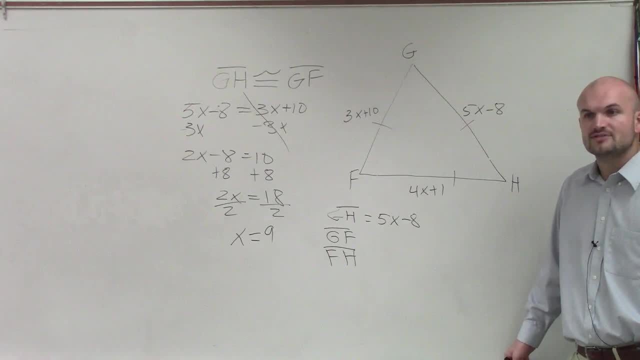 So gh equals 5x minus 8.. All right Now, Taylor. what does 8 equal? Good, So you can plug in 8 in for x. So it would be 5 times 8 minus 8.. So 5 times 8 is 40 minus 8 equals 32.. 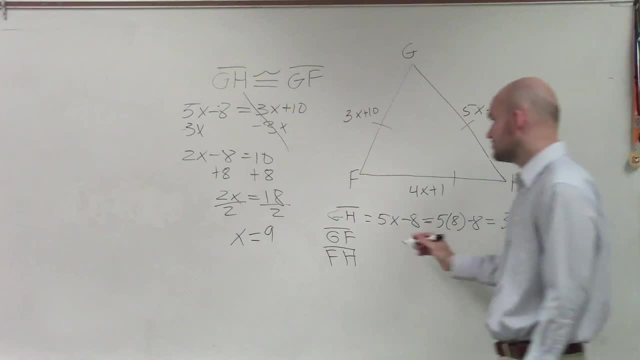 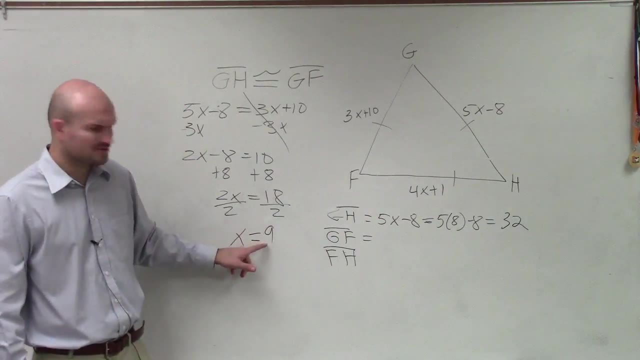 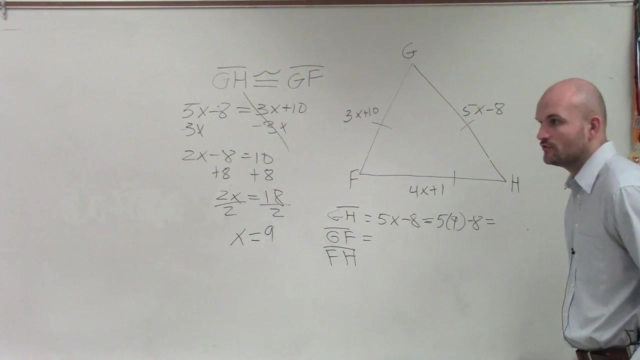 That means the measure of gh is 32.. Now let's do where I get what? Well, because it's 5 times x. Oh, x equals 9.. Thank you, Taylor. 5 times 9 is 45 minus 8 is going to be gf. 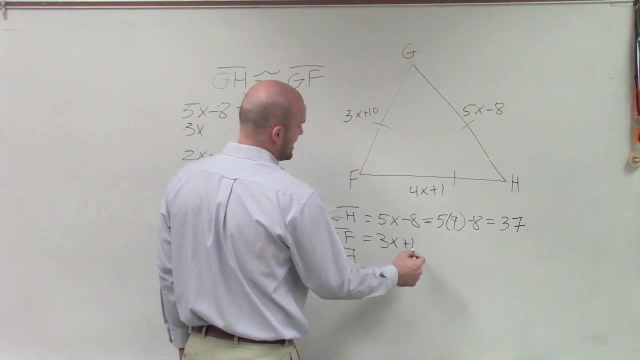 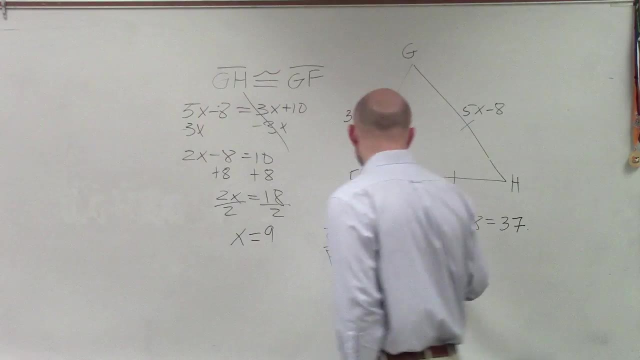 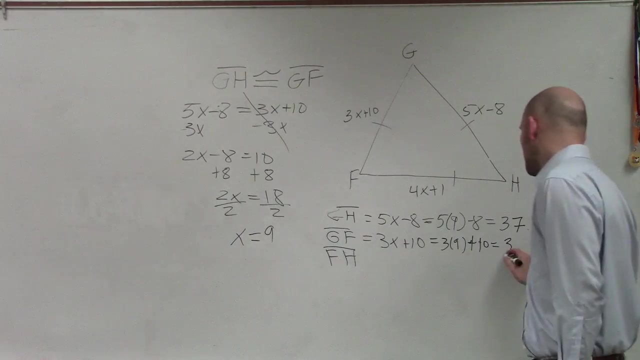 Now that's going to be 3x plus 10.. Well, remember Now remember, x equals 9.. So we do 3 times 9 plus 10. Which equals 37. Then we do fh, which is equal to 4x plus 1.. 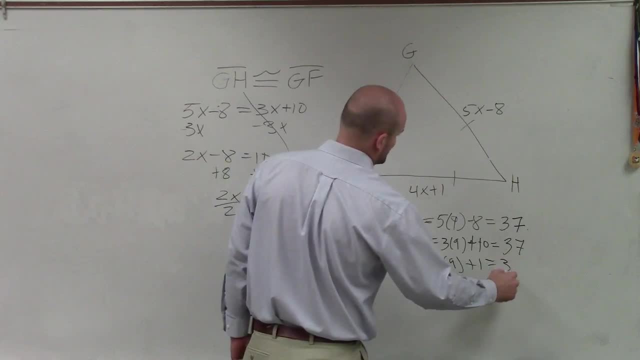 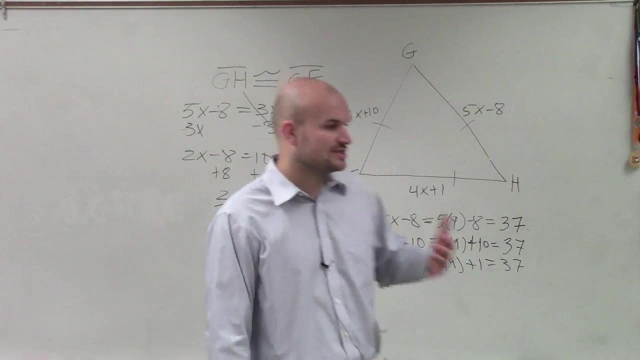 So that's 4 times 9 plus 1, which equals 37.. Okay, So you're really going to want to make sure, ladies and gentlemen, that when you're doing this you don't just solve for x, but you make sure you find the value of each side. 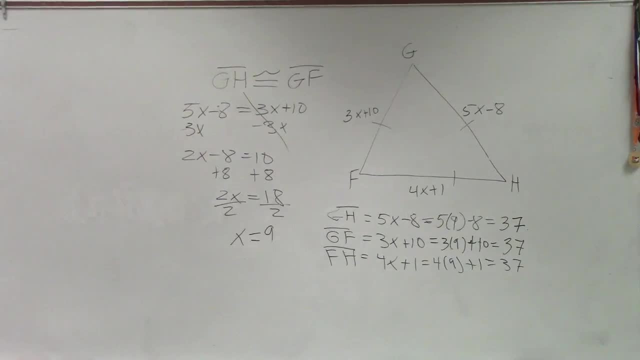 Yes, Colin, Go ahead. There's a little point there. There's a little point. I don't know why I leave it. Thank you.